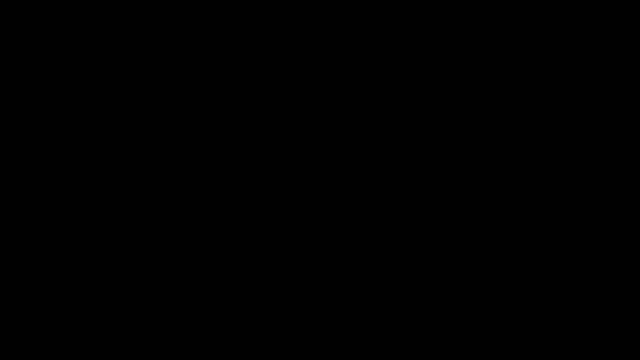 Now we're going to talk about two basic rules of probability. The first one is sometimes referred to as the addition rule. The probability of getting event A or event B can be written as the probability of A in union with B. This is equal to the probability of event A occurring. 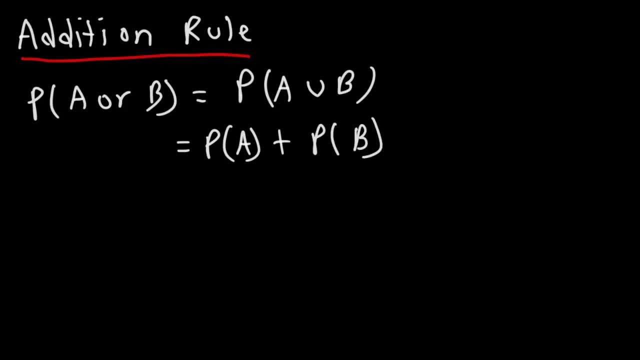 plus the probability of event B occurring, minus the probability of event A and event B occurring together. So make sure you know this Now. sometimes you may be dealing with two events that are mutually exclusive. For mutually exclusive events, the probability of getting event A and B together. 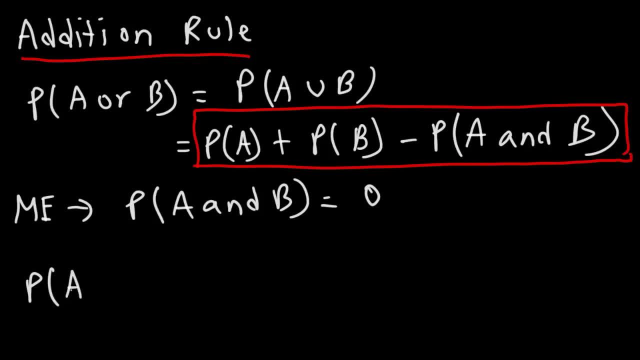 is zero. So therefore, the probability of getting A or B becomes P of A plus P of B if A and B are mutually exclusive events. But you can always use this formula, which will always work, regardless of what type of events you're dealing with. 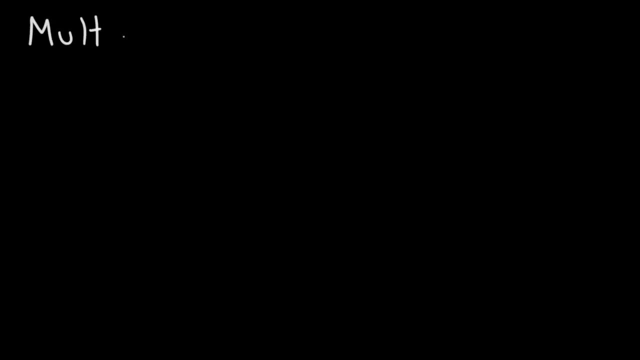 The next type of rule is the multiplication rule. So let's say if? well, first let's talk about conditional probability. The probability of A given B is the probability of getting A and B divided by the probability of getting B. So what this means is that if we multiply both sides by P of B, we can get this equation. 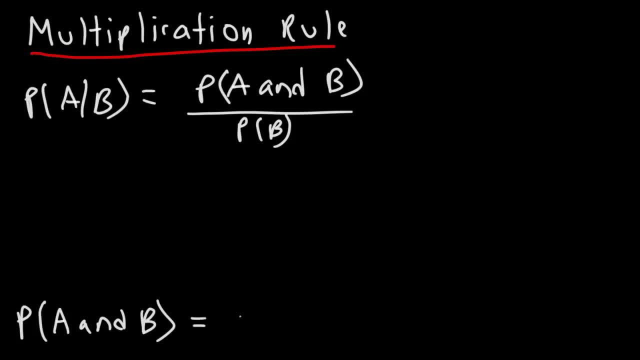 The probability of getting A and B is the product of the probability of getting A given B times the probability of event B occurring. Now what about this scenario? What is the probability of B given A? This is still the probability A and B occurring, but divided by the probability of A. So if we rearrange this equation by: 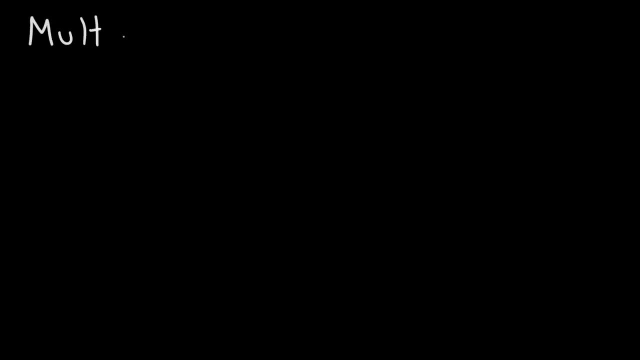 The next type of rule is the multiplication rule. So let's say if? well, first let's talk about conditional probability. The probability of A given B is the probability of getting A and B divided by the probability of getting B. So what this means is that if we multiply both sides by P of B, 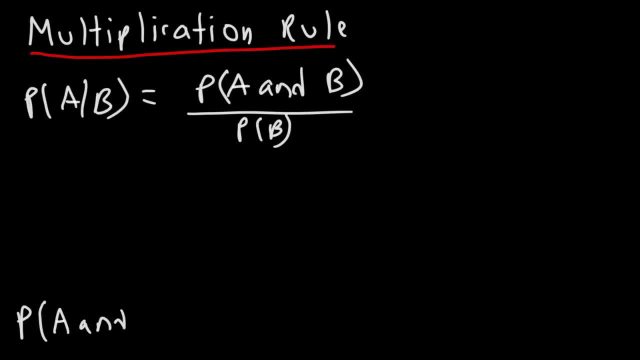 we can get this equation: The probability getting A and B is the product of the probability of getting A given B times the probability of event B occurring. Now what about this scenario? What is the probability of B given A? This is still the probability of A and B. 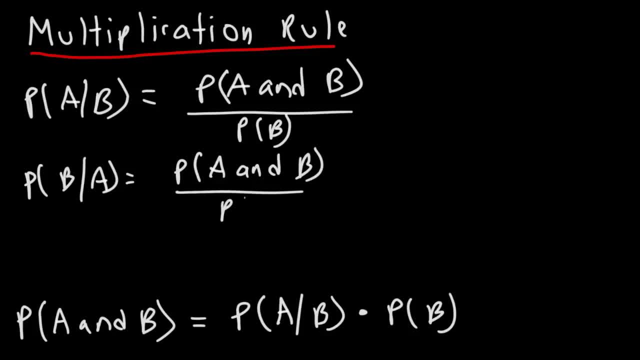 occurring, but divided by the probability of A. So if we rearrange this equation by multiplying both sides by P of A, we can see that the probability of A and B can also be written as the probability of B given A times the probability of A. So notice the similarities of these two. 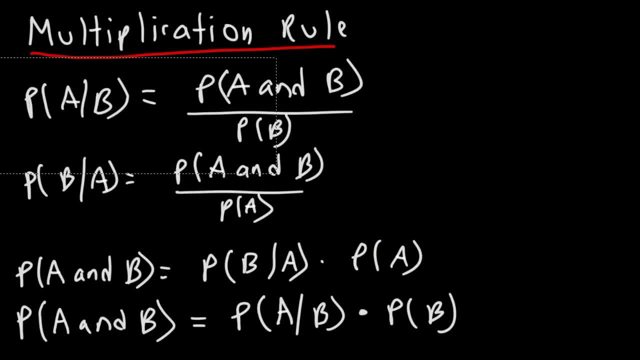 equations Now. sometimes the two events that you're dealing with might be independent events. An independent event is an event that does not depend on another event. For independent events, the probability of A given B is equal to the probability of event A occurring. 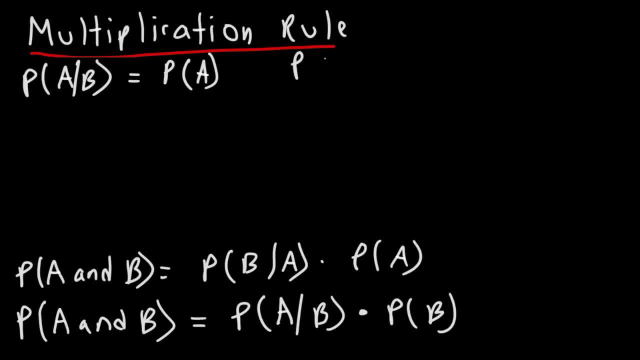 because A does not depend on B. Likewise, the probability of B given A is equal to the probability of event B occurring, because B does not depend on A. So when dealing with independent events, we get this equation: The probability of A and B occurring is simply the probability of A. 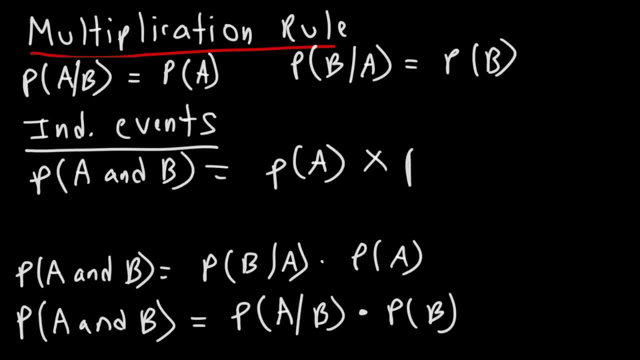 times, not plus, but times, the probability of A and B occurring. The probability of A and B occurring is similar with the probability of event B occurring. The probability of A and B occurring is not dependent on either of these two events, especially if the two events are independent. if not, 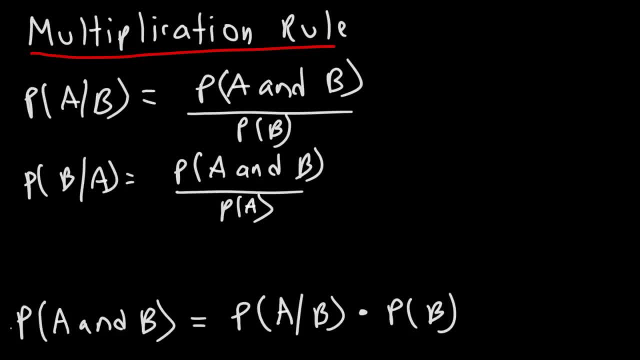 multiplying both sides by P, we can see that the probability of A and B can also be written as the probability of B given A times the probability of A. So notice the similarities of these two equations. Now, sometimes the two events that you're dealing with might be independent events. 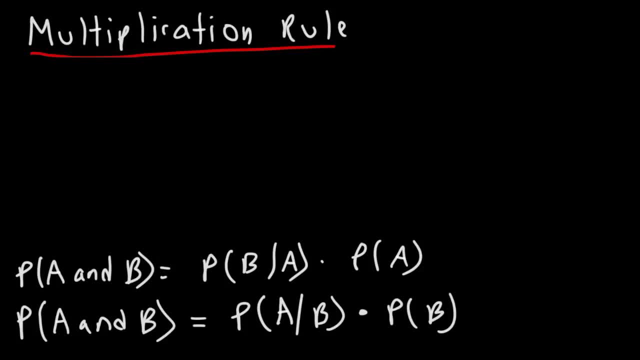 An independent event is an event that does not depend on another event. For independent events, the probability of A given B is equal to the probability of event A occurring, because A does not depend on B. Likewise, the probability of B given A is equal to the probability of event B occurring because 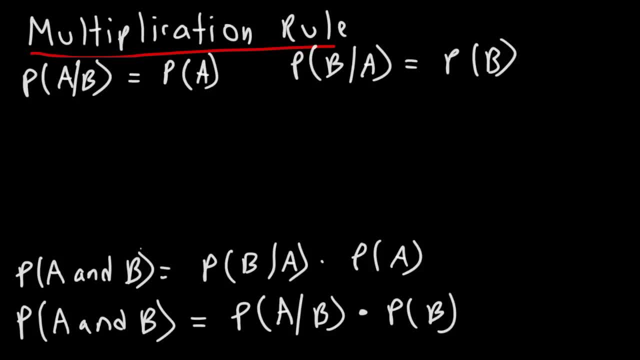 B does not depend on A. So when dealing with independent events we get this equation: The probability of A and B occurring is simply the probability of A times, not plus, but times the probability of event B occurring if the events are independent. 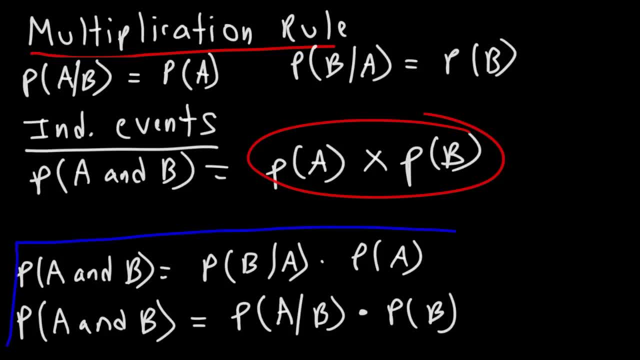 If not, then you can get one of these equations depending on what you're given. One thing I do want to mention is that when you see A and B occurring, this means that these two events are occurring at the same time. It doesn't mean A and then B, which could be different. 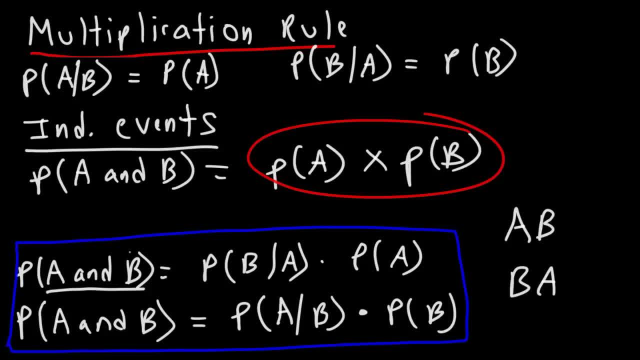 A and B are different from B and then A, So because the events occur at the same time, the order is not relevant. otherwise, the formulas may be affected. So just keep that in mind. Therefore, the probability of A and B occurring is the same as the probability of B and A. 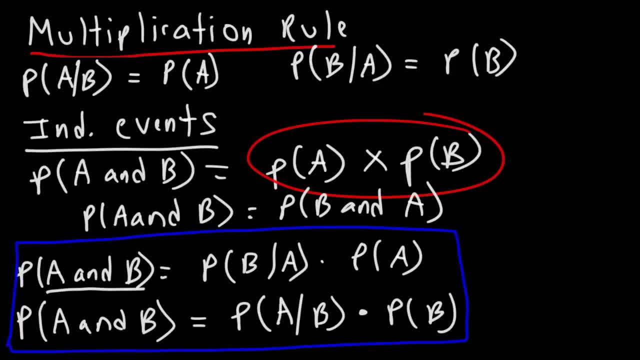 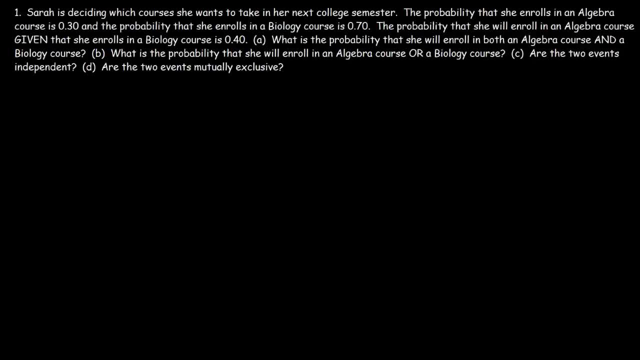 occurring because these two events occur at the same time, So I just want to add that clarification for those of you who may have questions on it. Now let's go ahead and put this information to good use. Sarah is deciding which courses she wants to take in her next college semester. 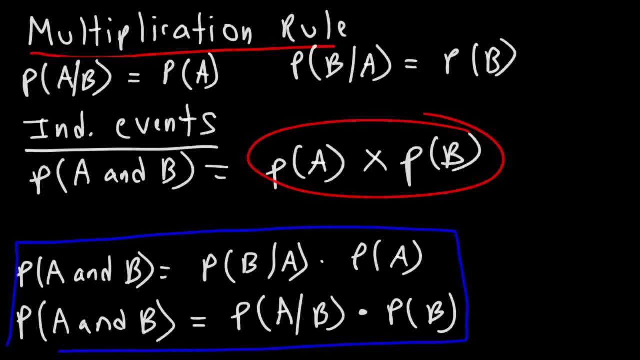 then you can get one of these equations. depending on what you are given When dealing with independent events, you can get one of these equations. One thing I do want to mention is that when you see A and B occurring, this means that these two events are occurring at the same time. It doesn't mean A and then B. which could be different from B and B. if we look at the momentum, the diagram is getting Okay, so that feels good. and now we will be looking for our feminist governing method- ie video right. we will be looking for our feminist governing method- ie Jeong's method- ie video right. 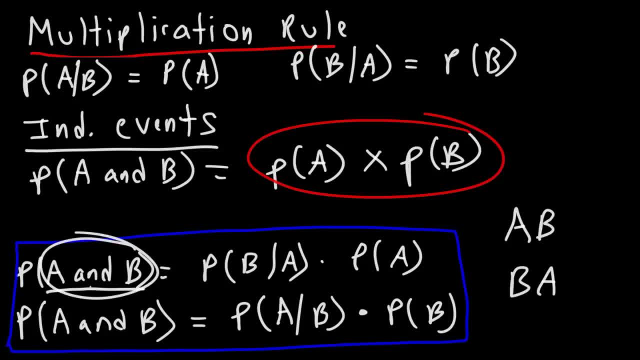 B and then A. So because the events occur at the same time, the order is not relevant. Otherwise the formulas may be affected, So just keep that in mind. Therefore, the probability of A and B occurring is the same as the probability of B and A occurring because these two events 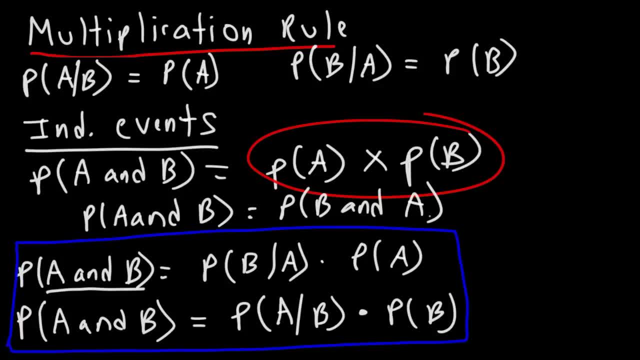 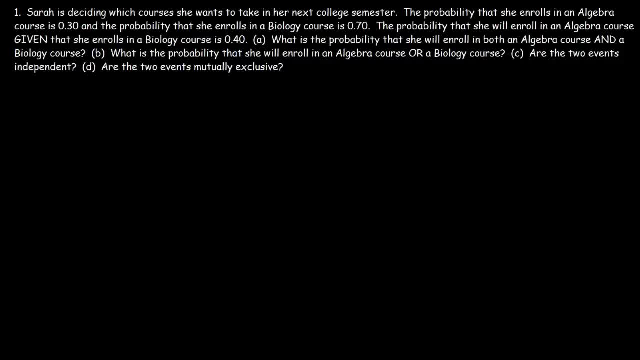 occur at the same time. So I just want to add that clarification for those of you who may have questions on it. Now let's go ahead and put this information to good use. Sarah is deciding which courses she wants to take in her next college semester. The probability that she enrolls in. 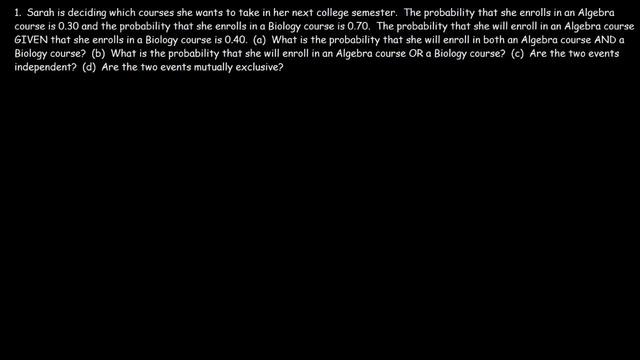 an algebra course is 0.30, and the probability that she enrolls in a biology course is 0.70.. The probability that she will enroll in an algebra course, given that she enrolls in a bio course, is 0.40.. So, part A, what is the? 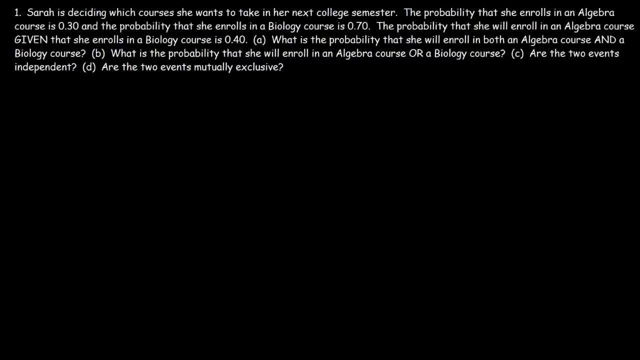 probability that she will enroll in both an algebra course and a biology course. So take a minute, pause the video and, using the formulas that we discuss, go ahead and get the answers to these questions. So first, let's begin by writing down what we 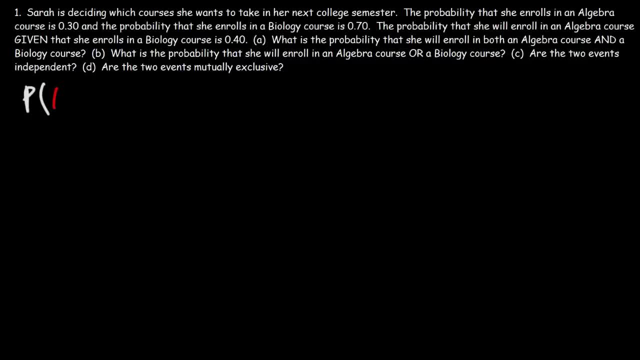 know, The probability that she takes an algebra course, that is, P of A, is 0.30.. And the probability that she takes a bio course, that's 0.70.. Now the probability of A given B, that is, that she takes an algebra course, given that she takes a bio course, 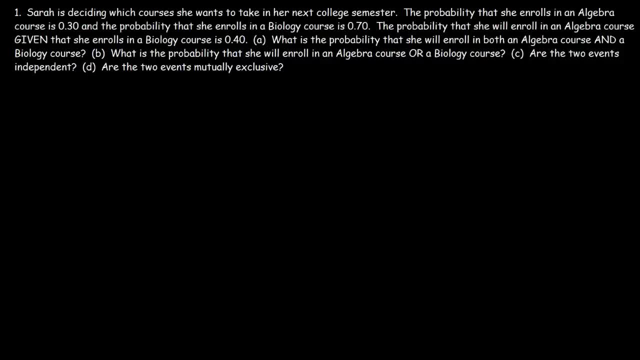 The probability that she enrolls in an algebra course is 0.30, and the probability that she enrolls in a biology course is 0.70.. The probability that she will enroll in an algebra course, given A and B occurring, is: 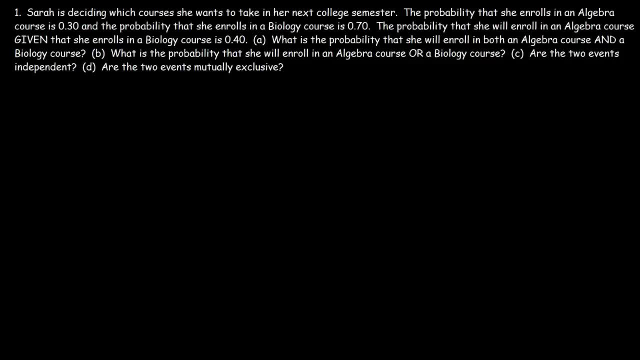 0.30.. The probability that she enrolls in a bio course is 0.40.. So, part A, what is the probability that she will enroll in both an algebra course and a biology course? So take a minute, pause the video and, using the formulas that we discuss, go ahead and. 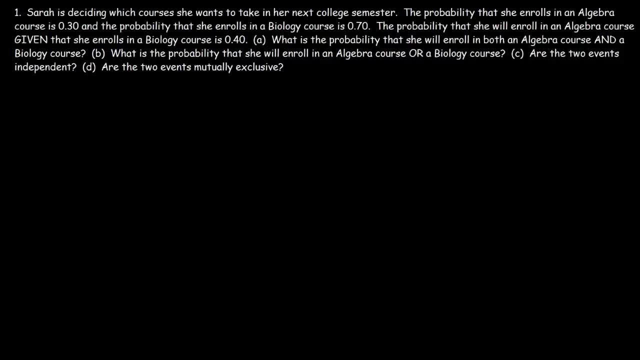 get the answers to these questions. So first let's begin by writing down what we need. So first let's begin by writing down what we need. So first let's begin by writing down what we need: watching and receiving. Here we can情. 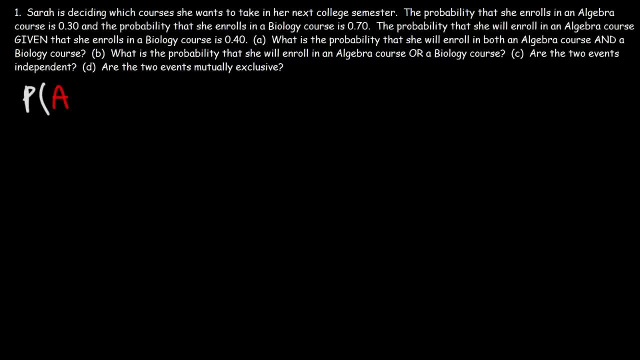 大 摬. the probability that she takes an algebra course that is P is 0.30, and the the probability that she takes an algebra course that is P is 0.30, and the probability that she takes an algebra course that is 0.70.. 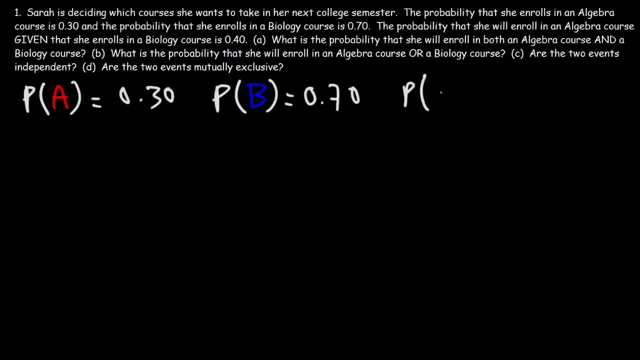 BE CAREFUL. Now the probability of A given B, that is, that she takes an algebra course. given that she takes an algebra course, that is already basic A, That's the absolute, That's off 0.40.. So with this information we can now focus on part A. So we're looking for the 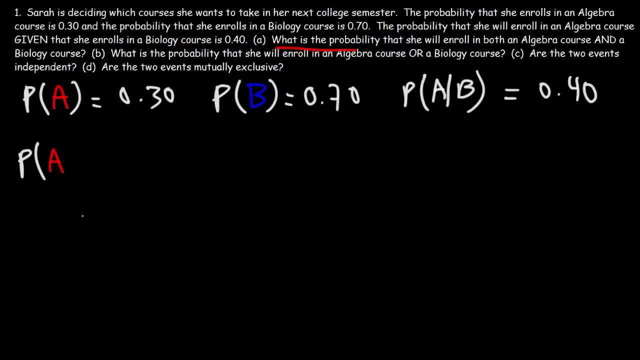 probability that she will take both algebra and bio. So what's the formula for this? This is equal to the probability of A given B times the probability of event B occurring. So we can see that P of A given B is 0.40.. And the probability that she will take a bio course. 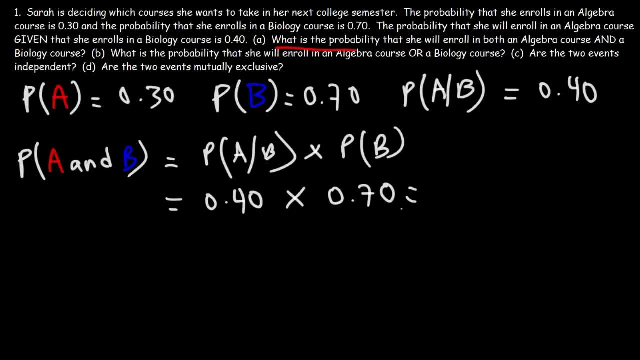 is 0.70.. Now 4 times 7 is 28.. So 0.4 times 0.7 is 0.28.. So there's a 28% chance that she's going to take both algebra and biology. Now let's move on to part B. What is the probability? 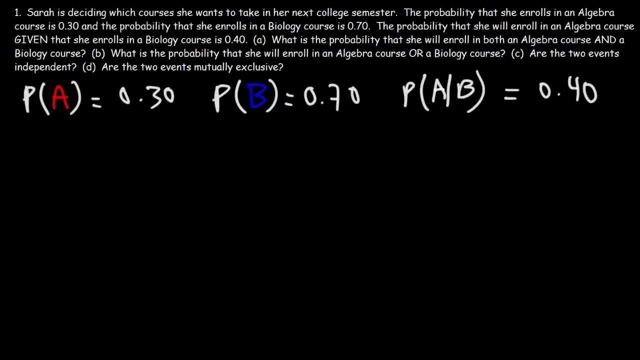 that's 0.40.. So with this information we can now focus on part A. So we're looking for the probability that she will take both algebra and bio. So what's the formula for this? This is equal to the probability of. 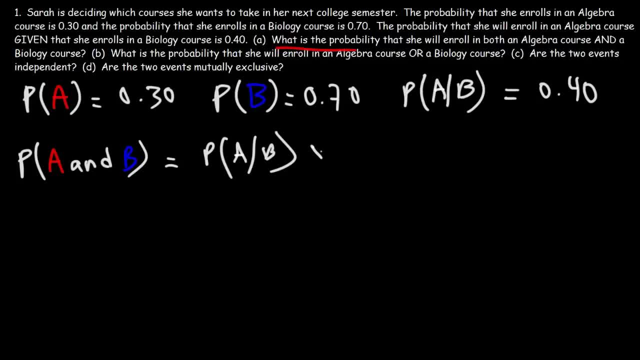 A taking an algebra course. that is P of A given B. that is P of A A given B times the probability of event B occurring. So we can see that P of A given B is 0.40.. And the probability that she will take a bio course is 0.70.. Now, 4 times 7 is 28.. 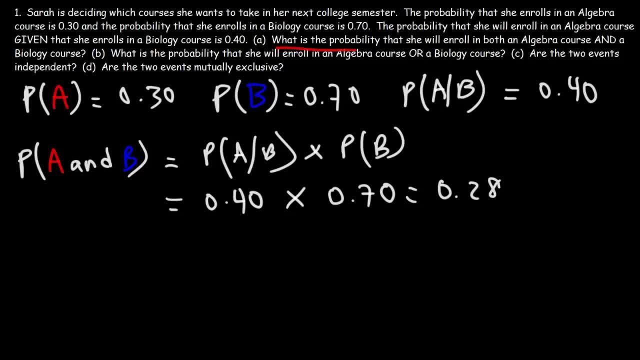 So 0.4 times 0.7 is 0.28.. So there's a 28% chance that she's going to take both algebra and biology. Now let's move on to part B. What is the probability that she will enroll in an algebra course or a biology course? 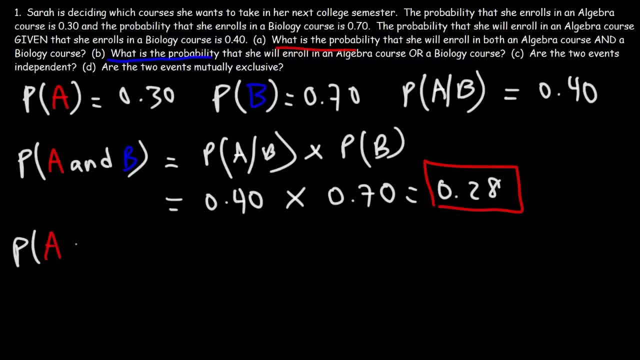 So this time we're looking for P of A or B. So what's the formula for this? So this is going to be based on the addition rule as opposed to the multiplication rule. So this is P of A plus P of B, minus P of A and B. 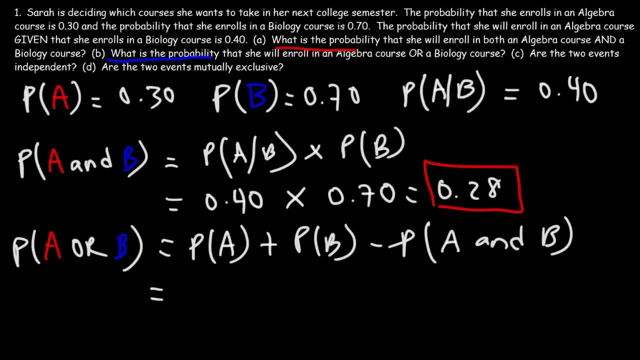 Now the probability that event A will occur is 0.3.. And the probability that she's going to take the biology course is 0.7.. The probability that she will take both algebra and biology- we have it here That- is 0.28.. 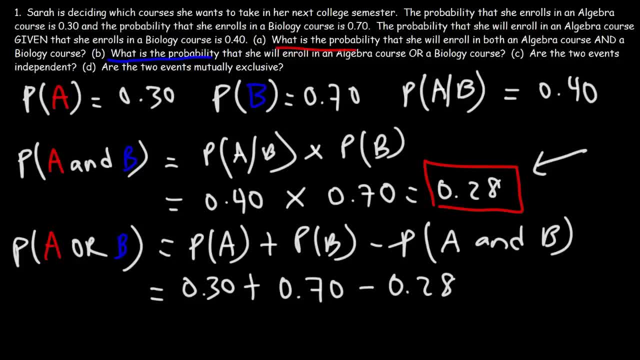 So let's go ahead and subtract these numbers, So 0.3 plus 0.7 minus 0.28.. This is equal to 0.72.. So there's a 72% chance that she will take algebra or biology. Now let's move on to part C. 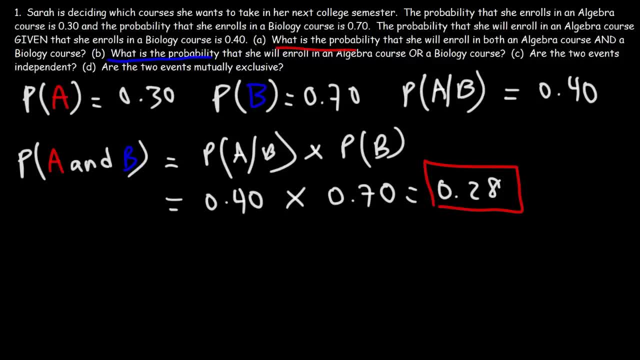 that she will take a bio course. So we can see that P of A given B is 0.40.. And the probability that she will enroll in an algebra course or a biology course. So this time we're looking for P of A or B. So what's the formula for this? So this is going to be based on the addition rule. 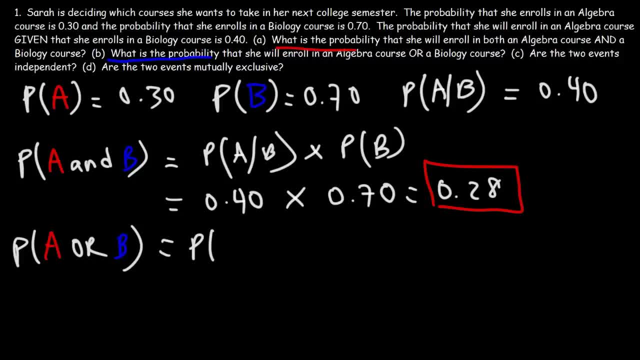 as opposed to the multiplication rule. So this is P of A plus P of B, minus P of A and B. Now the probability that event A will occur is 0.3.. And the probability that she's going to take the biology course is 0.7.. The probability that she will take both algebra 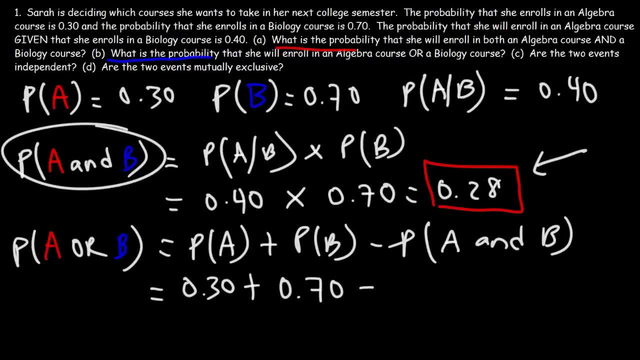 and biology. we have it here, That is 0.28.. So let's go ahead and subtract these numbers So 0.3.. 0.3 plus 0.7 minus 0.28. This is equal to 0.72.. So there's a 72% chance that she will take algebra. 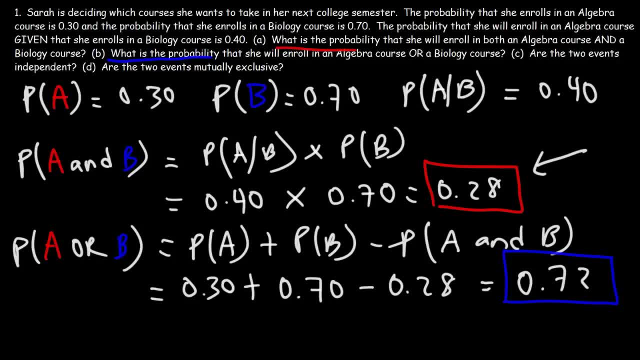 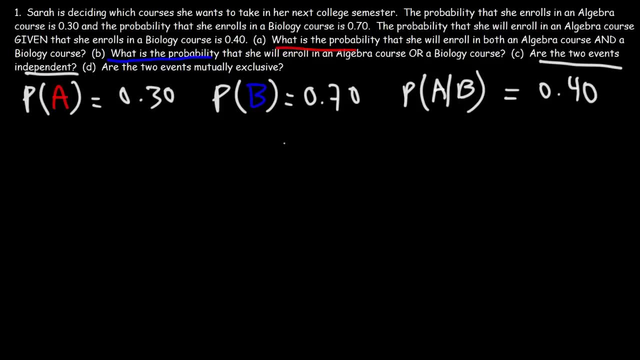 or biology. Now let's move on to part C. Are the two events independent? What would you say? Okay, What are the requirements for two events to be independent? In order for events A and B to be independent, the probability of A given B must be equal. 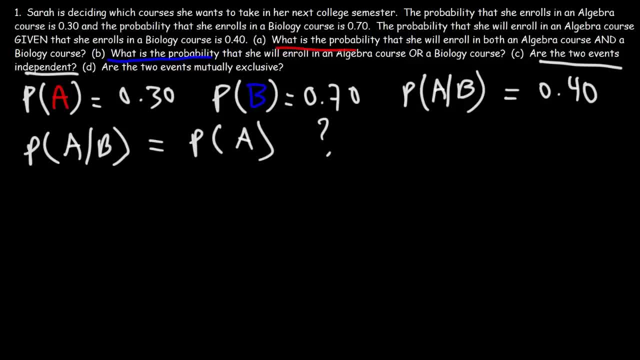 to the probability of A. Are they equal? The probability of A given B, we could see that it's 0.4.. And the probability of event A occurring is 0.3.. So these two are not equal. Therefore, the two events are not independent of each other. 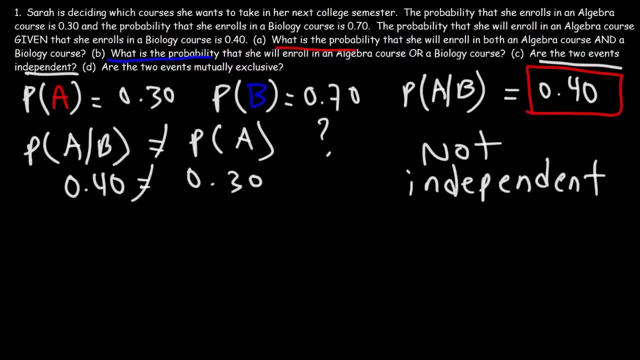 Now, what about part D? Are the two events mutually exclusive? What would you say? In order for the two events to be mutually exclusive, the probability of event A occurring and event B occurring must be equal to 0.. Is this true? Well, we know that A and B the probability.